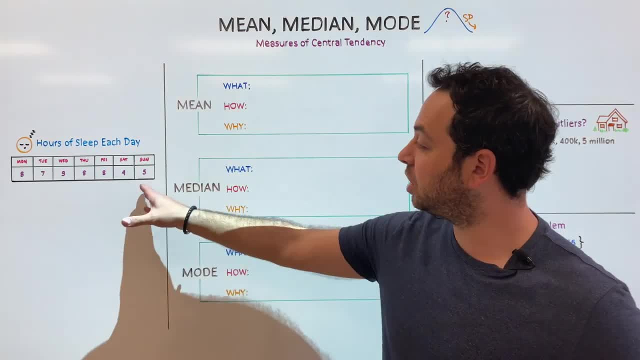 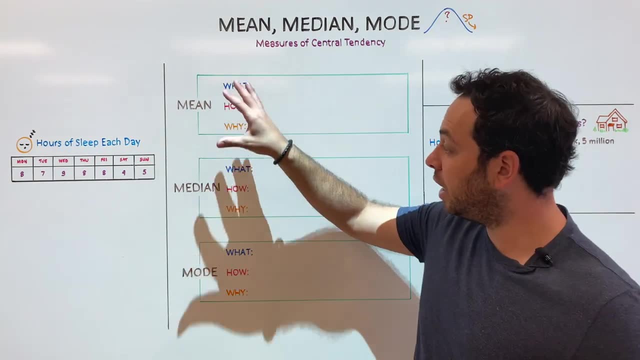 hours. On Thursday you slept a total of eight hours And on Sunday you slept a total of five hours. And you just want a better understanding of your sleep patterns? Well, guess what The mean, the median and mode can help you. 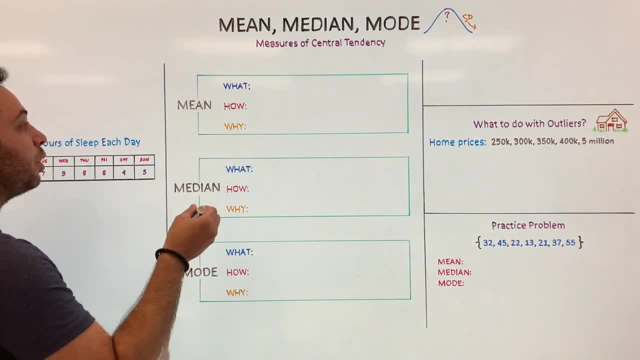 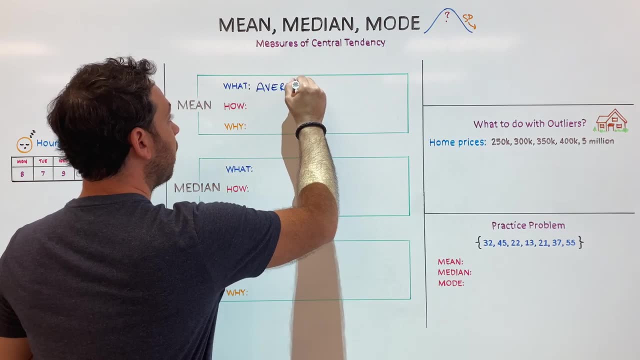 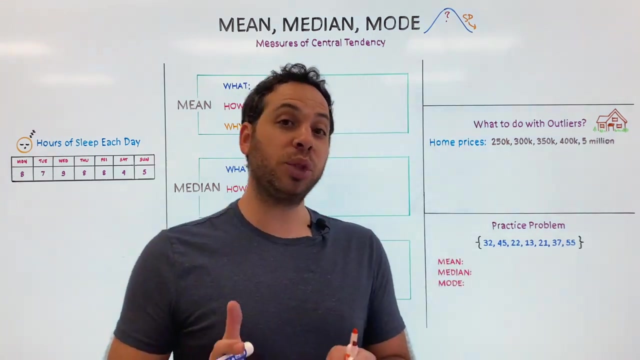 Let's start with the mean, the what, the how and the why. Let's start with the what. The mean is what we consider: the average or the arithmetic average. All right, This is probably the most common measure of central tendency that we use And, by the way, you might not have used the word mean, but you've. 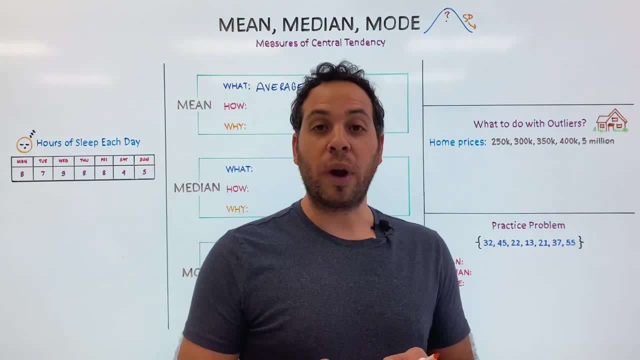 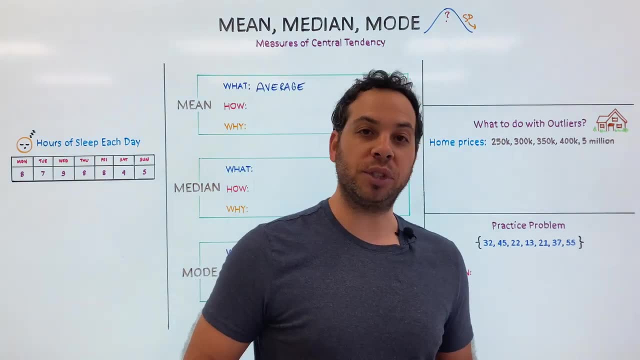 calculated it many times in your life. For example, if you rent an apartment or you own a house and you're trying to find out the average monthly cost of electricity or gas or cable- you have used the mean. Or if you follow sports and you want to know a baseball player's batting average or a basketball 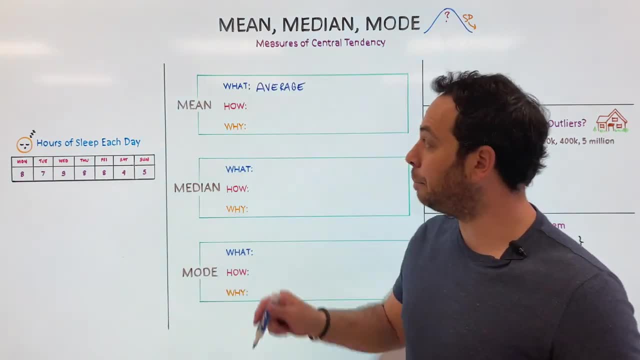 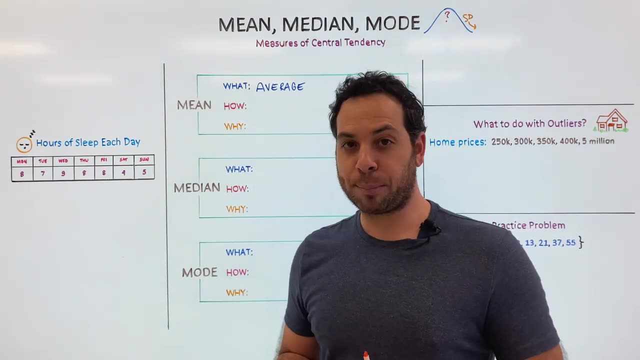 player's average points per game. you have not used the word mean, but you are calculating the mean. So there's some interesting information. Now, how do we calculate the mean? There's a two-step process. The first thing we do is we add up each individual data point. each one represents a data. 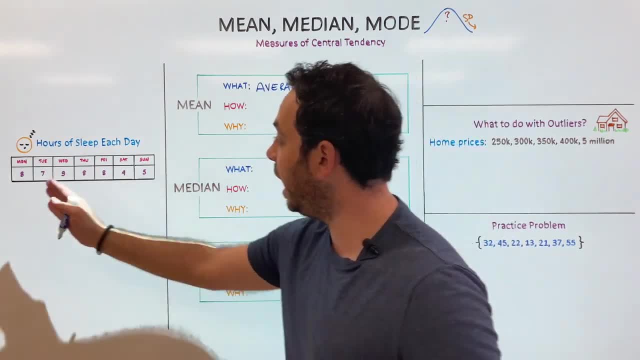 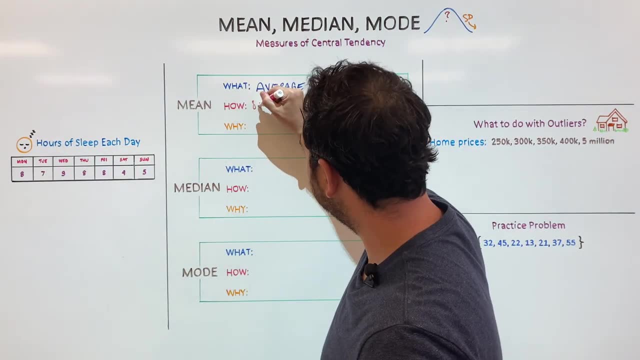 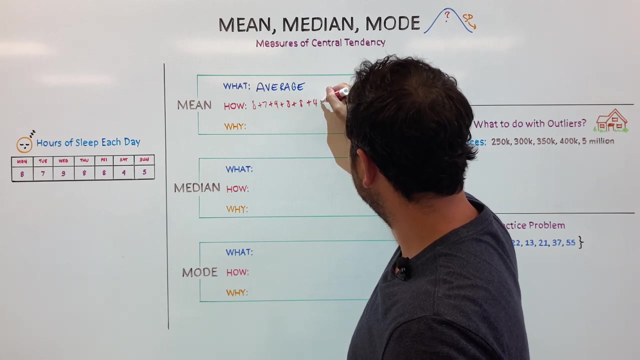 point in our data set. So let's do that together: Eight plus seven plus nine plus eight plus eight plus four plus five. Let's do that together: We have eight plus seven plus nine plus eight plus eight plus four plus five. All right, What does? 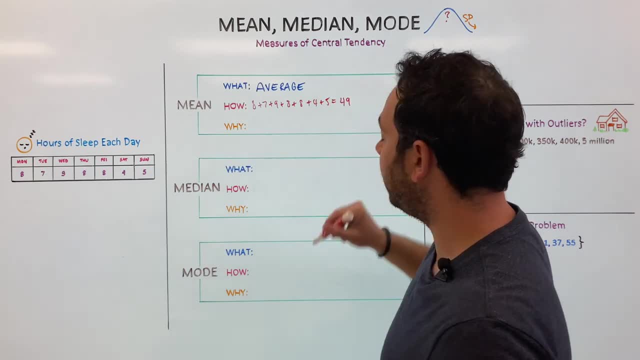 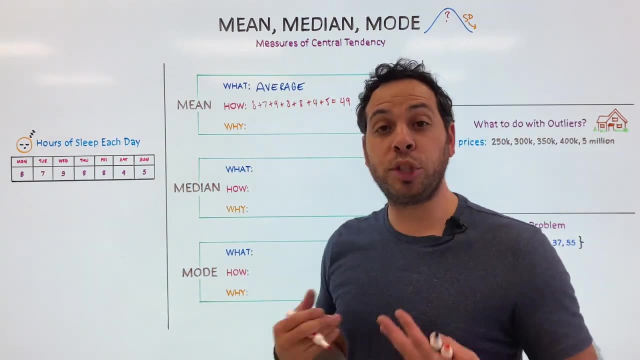 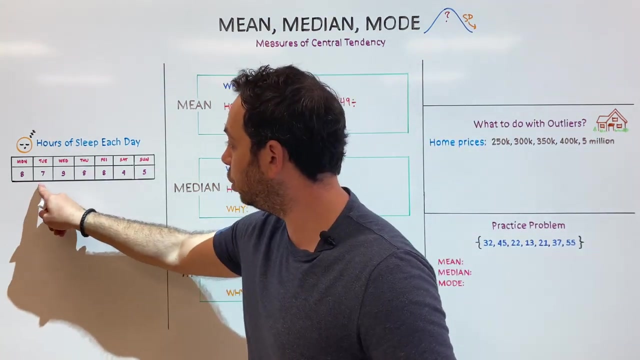 that equal, That's going to equal 49. That becomes our sum. So that's step one. Add up each individual data point to get your sum. And then what do we do with our sum? We divide our sum by the total numbers in our data set. How many are there? One, two, three, four, five, six, seven. Divide by seven. 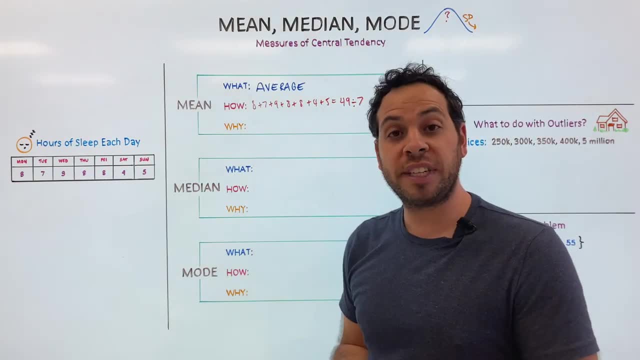 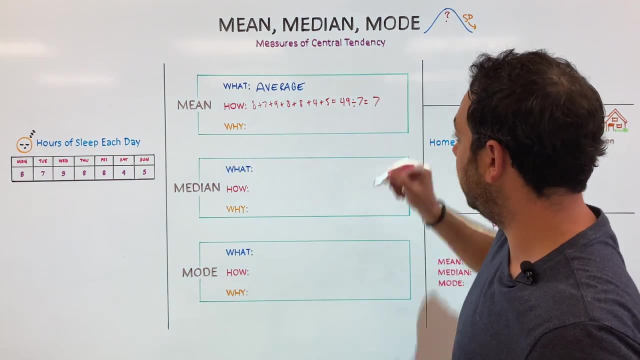 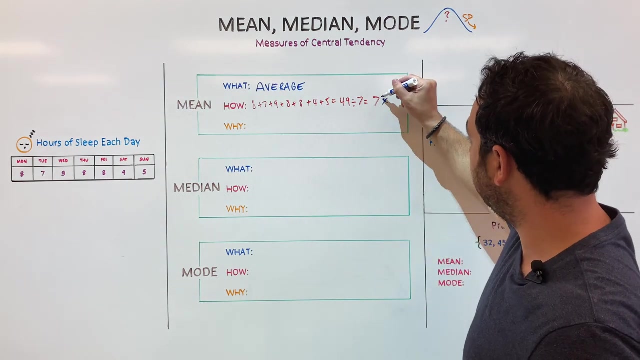 So we take our sum, divide by the total number of data points in our data set and the answer becomes our mean. Forty-nine divided by seven is seven And that becomes our mean. And, just as a side reference, this is our symbol for the mean. Okay, So our seven is the mean. Now why would you use the mean over? 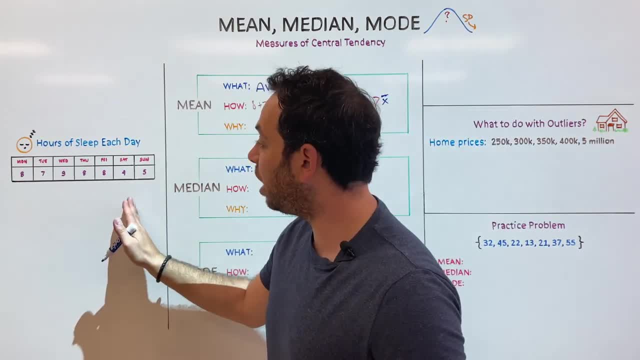 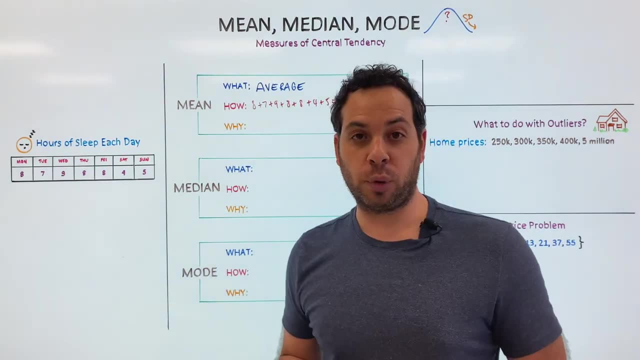 the median and the mode. Well, if you look at our data points, because they are relatively the same, the mean is the best measure of central tendency to use. If you had an outlier, for example, an outlier is a score that is so far away from each individual data point the mean would not. 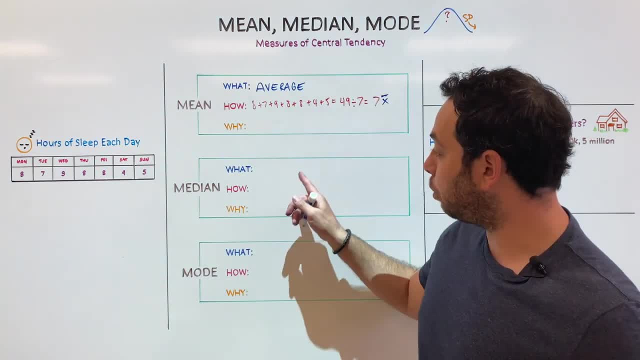 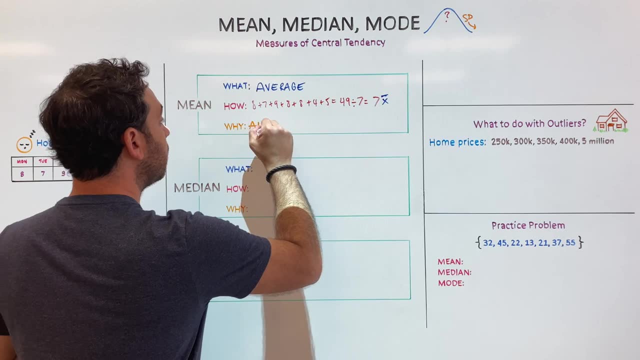 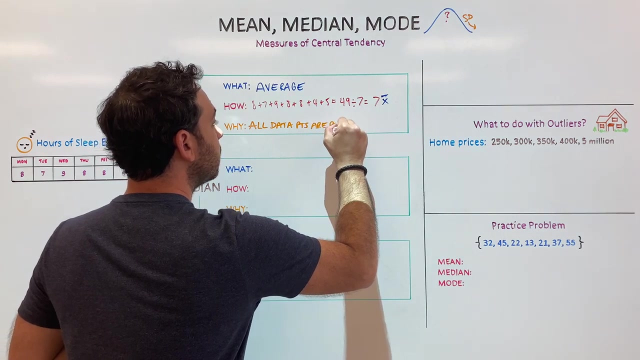 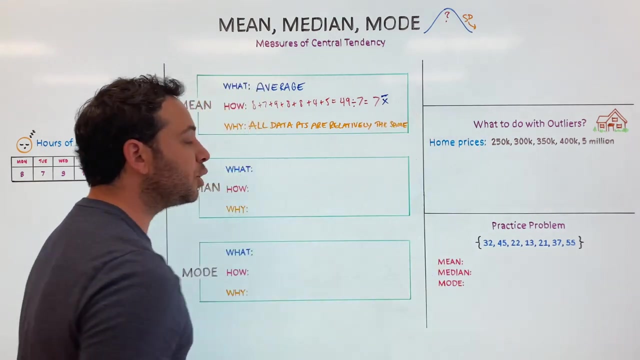 be the best measure of central tendency to use, And we'll talk about outliers more when we get to median, So let's write it together. Why would we use the mean When all the data points, all the data points, are relatively, relatively the same? Okay, All right, So let's move on to our next measure of. 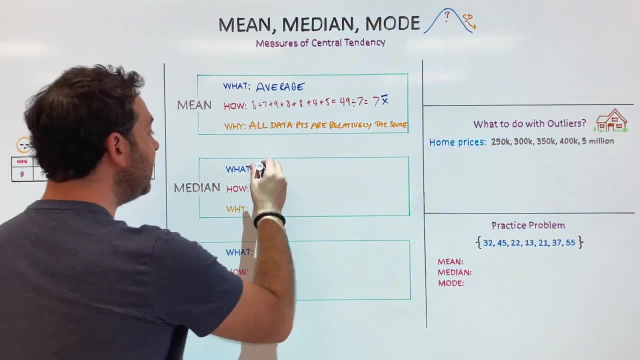 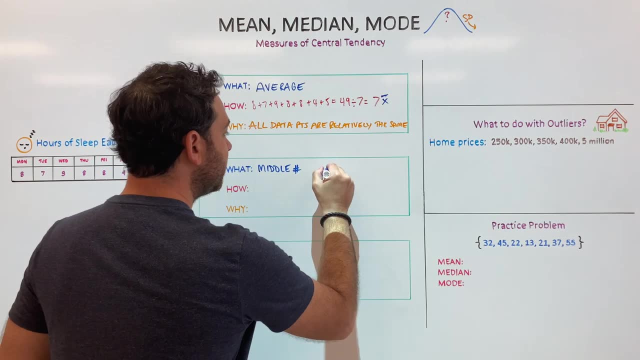 central tendency: the median. What is the median? The median represents our middle value or middle number. All right, In other words, if this dot is our median, we are going to have 50% of our data points going in one direction. 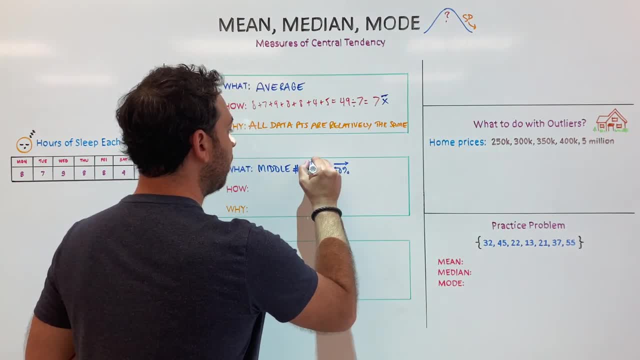 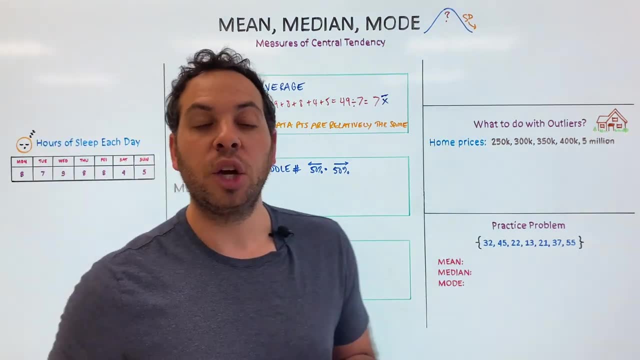 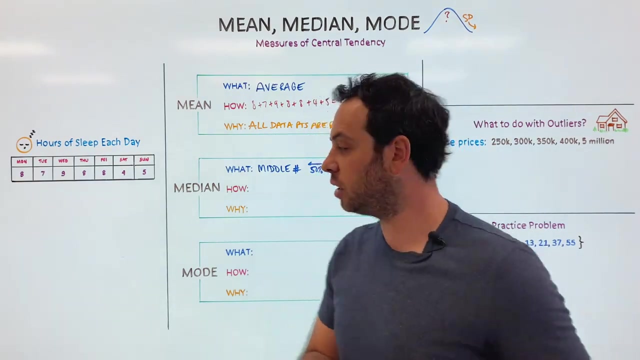 and 50% of our data points going in the other direction. What's the middle, Our median. Now, how do we actually find our median? We put our numbers in our data set in numerical order, from least to most, from lowest to highest. So let's do that together. Our lowest would be: 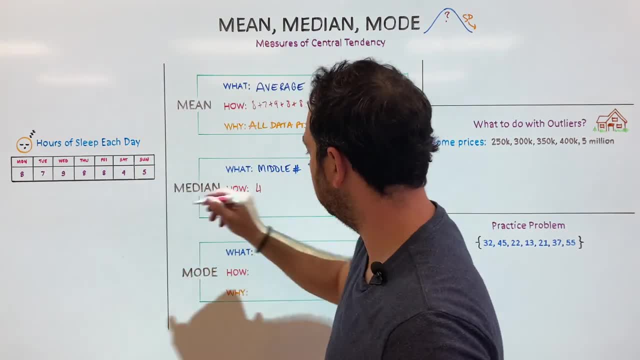 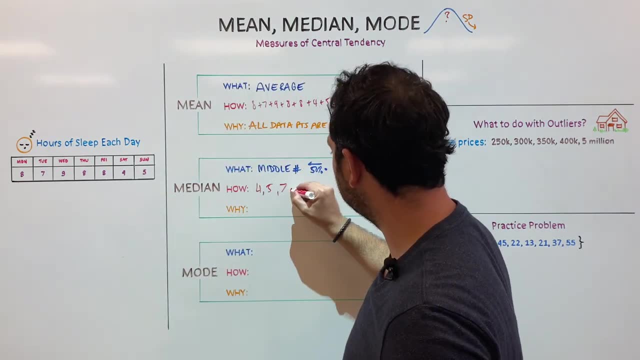 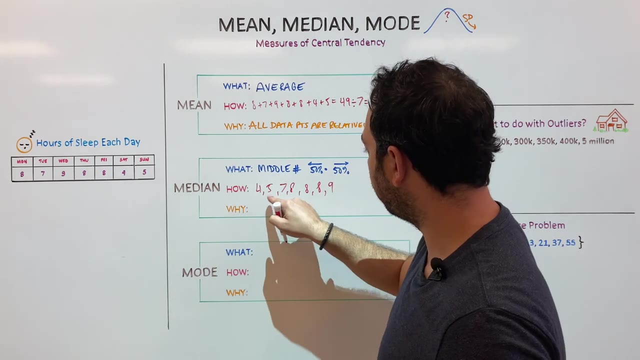 find it with me- four, then five, then seven, And look, we have a few eights: one, two, three, So eight, eight, eight, And then, finally, our highest number would be nine. Okay, So we go four. 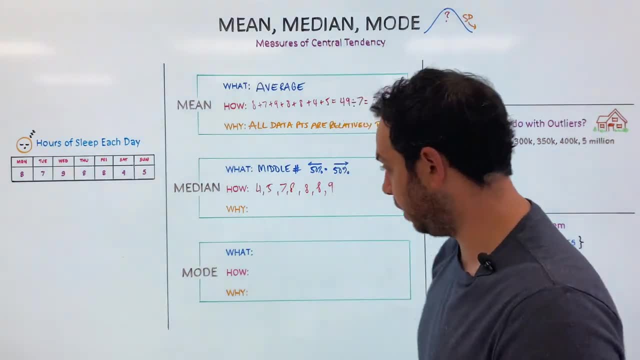 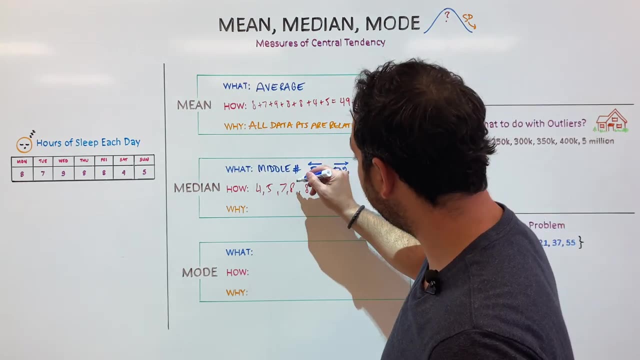 five, seven, eight, eight, eight, nine. Now, where is our median? Well, our median has to be in the middle, where 50% is in one direction and 50% is in another direction. And through that logic, 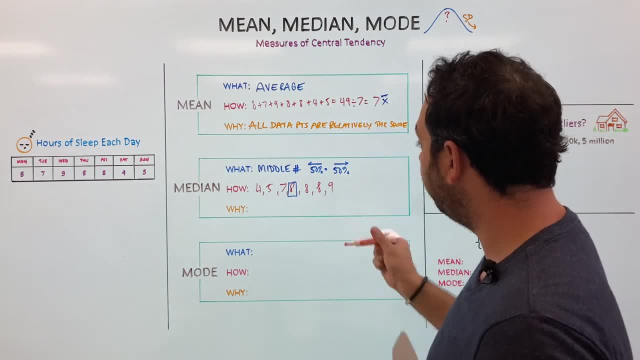 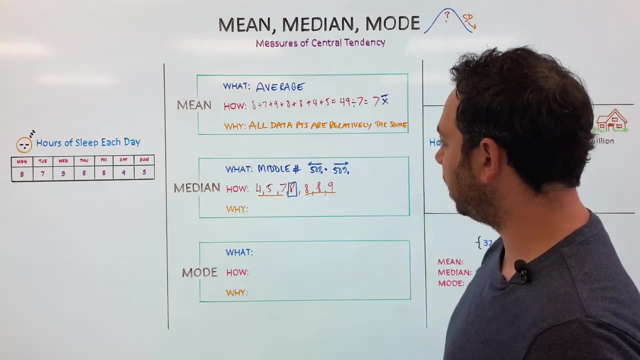 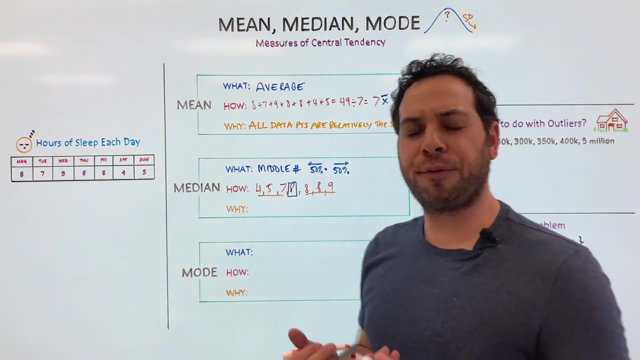 eight- right here would be our median, because I know we have three digits going in this direction and three digits going in that direction, 50% here and 50% here. So the median would be eight. Now you'll notice there's an odd number, But how do you find the? 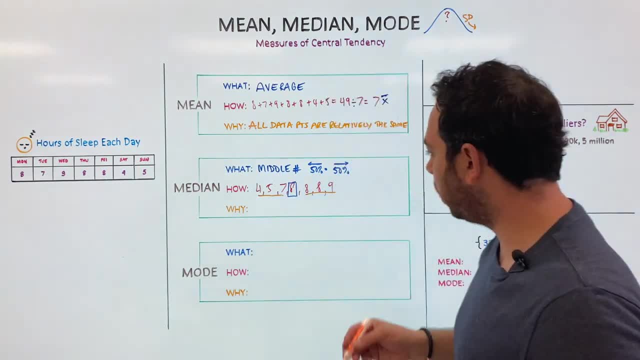 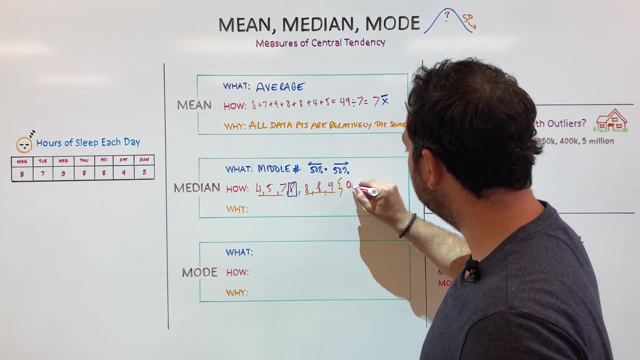 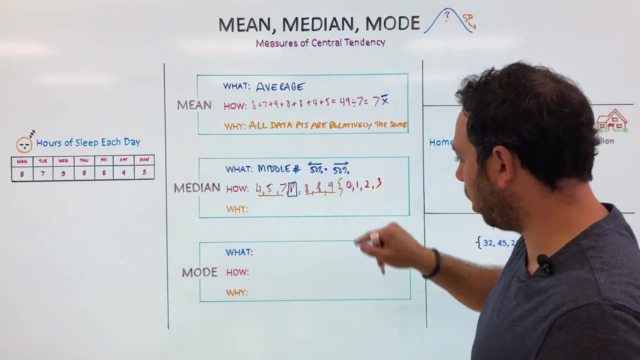 median if there are even numbers. Well, let's think about this together. Okay, Let's imagine that our numbers are zero: one, two, three. Where's our median Right? There is no middle number. So what do we do? Well, the next best thing to do is we take 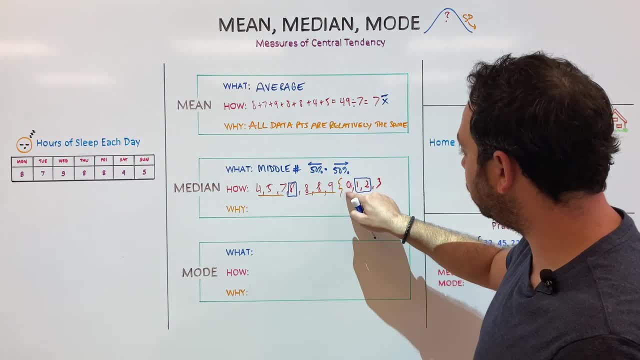 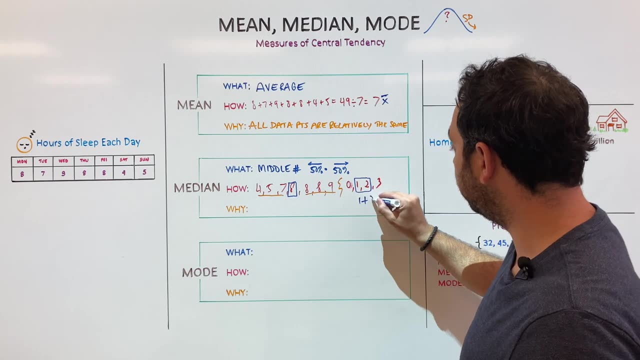 two middle numbers — and I know these are two middle because I had one digit here, one digit here, right, 50% here, 50% there — we add them together, right. one plus two equals three, and then we divide it by two because we have two. 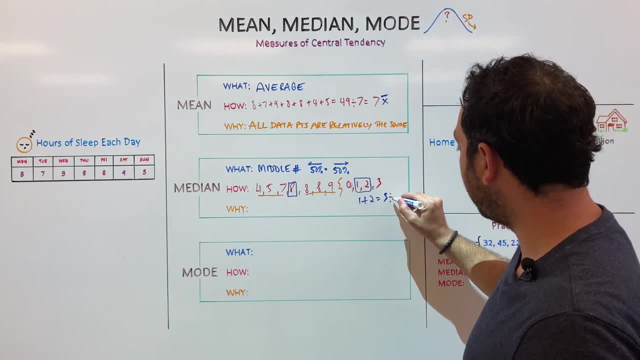 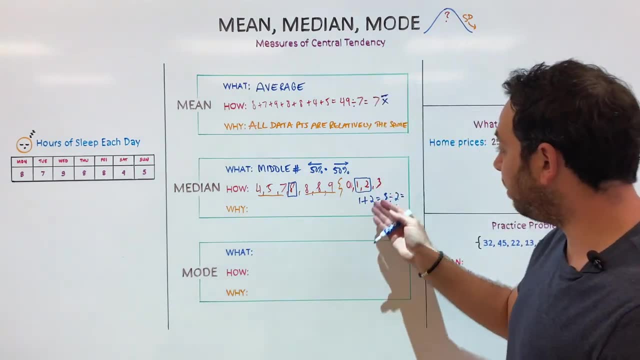 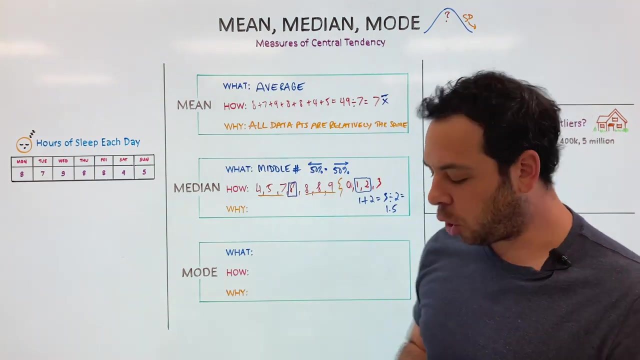 digits — one, two. So we have three divided by two equals 1.5. And 1.5 becomes our median when we have an even number. So there's our median median versus, let's say, the mean or the mode we would use a median when we have. 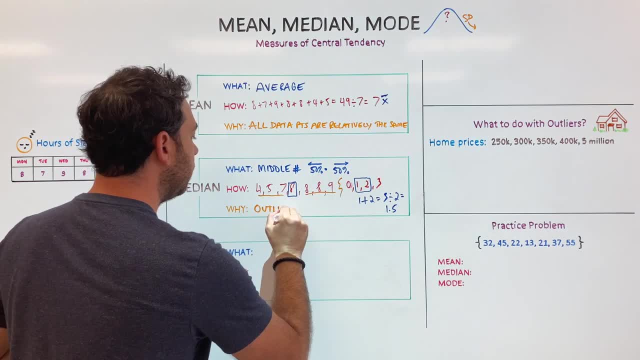 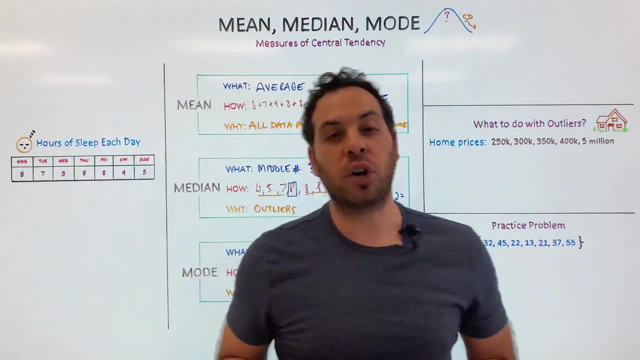 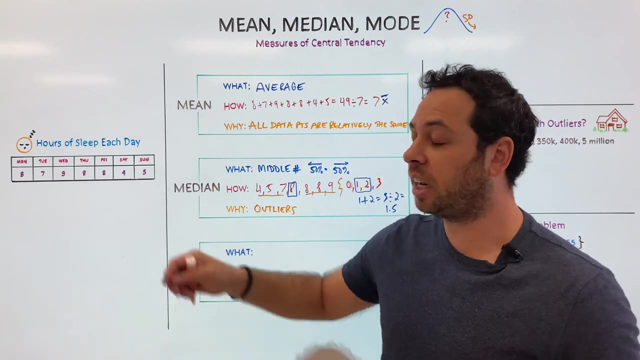 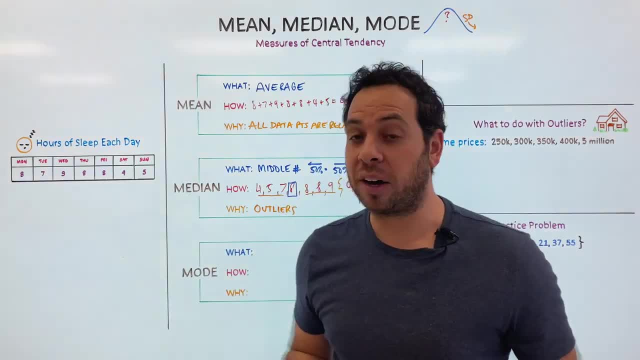 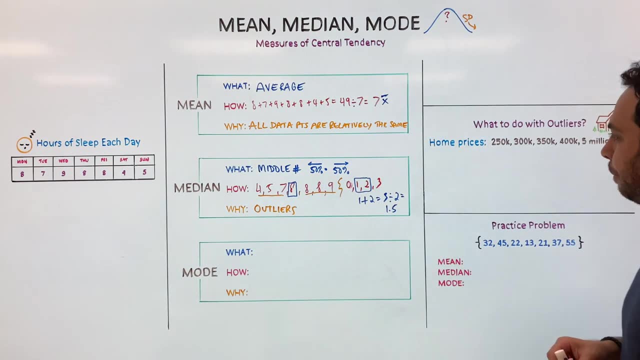 zero hours? well, zero would be an outlier because it's so far away than the other data points. so what do we do? well, let's do an example together, okay, and we're going to do a little error here to show you that we're moving up to here. what do? 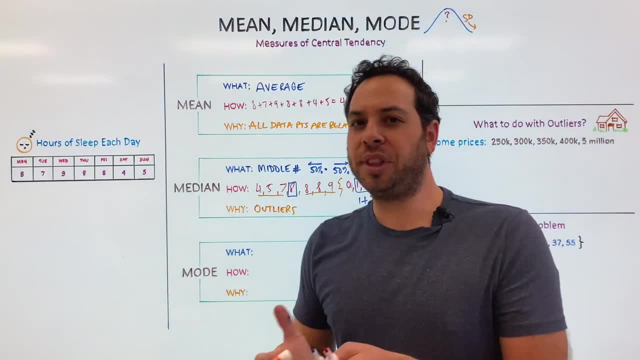 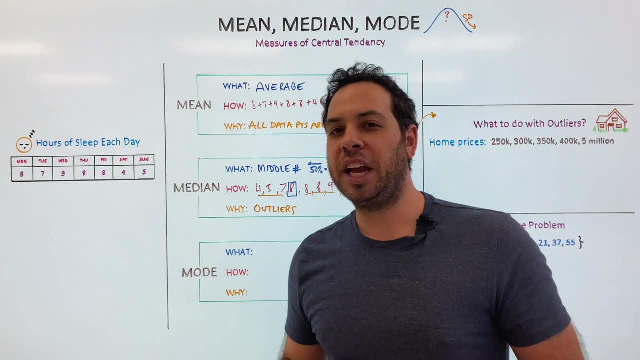 we do with outliers. in other words, why wouldn't we use the meat? let's do this together. let's imagine we are looking for homes, okay, and you're moving to an area and you like it in, your family likes it, and you happen to pick a random sample of five homes. here are the prices. 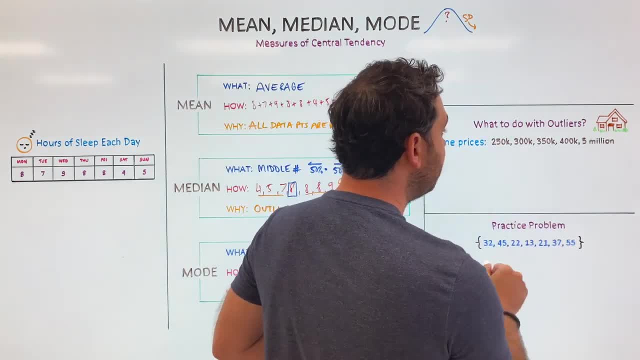 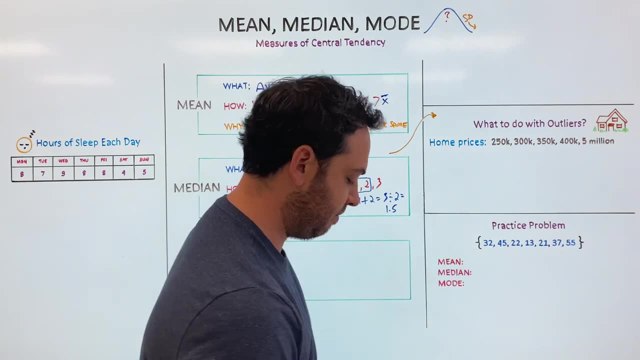 250,000, 300,000, 350,000, 400,000 and 5 million, And you're like, I'm just going to calculate the mean to see if I can live there. So how do we calculate the mean? Remember the two-step process. First, we add up each data. 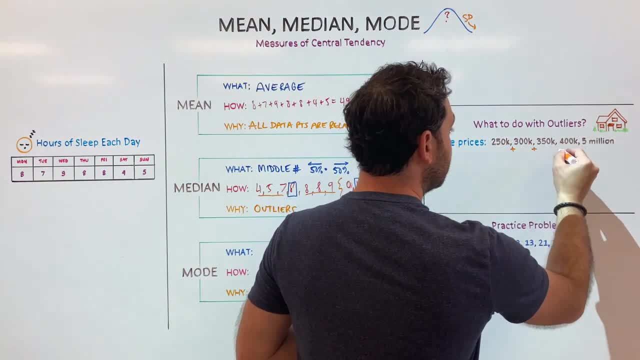 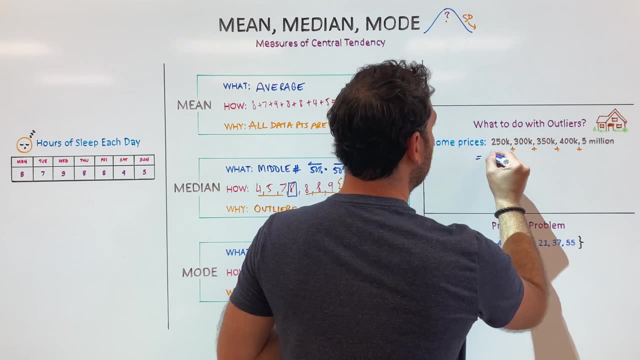 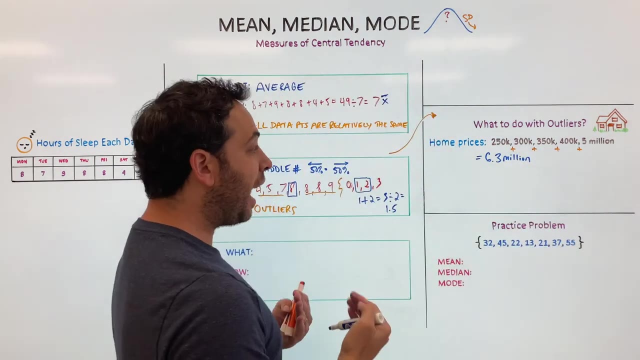 point: 250,000 plus 300,000 plus 350,000 plus 400,000 plus 5 million- I've never done this calculation before- This is going to equal $6.3 million. Now what do we do? We divide that. 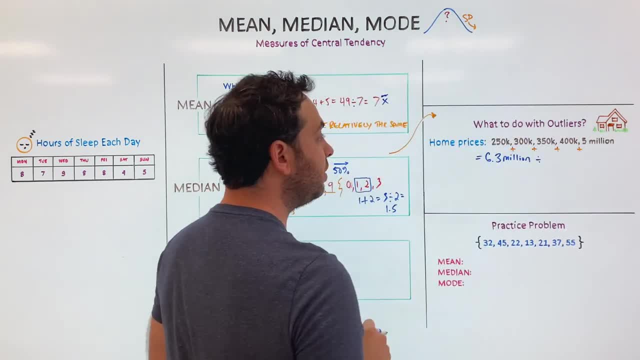 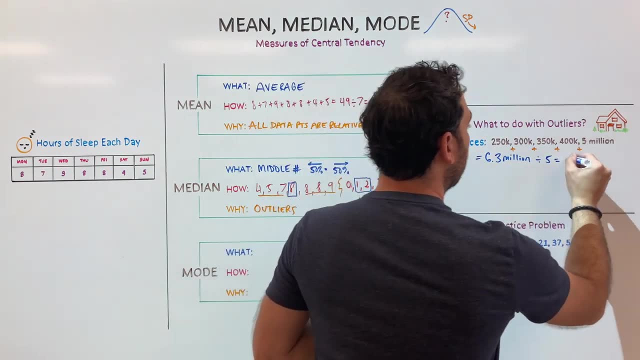 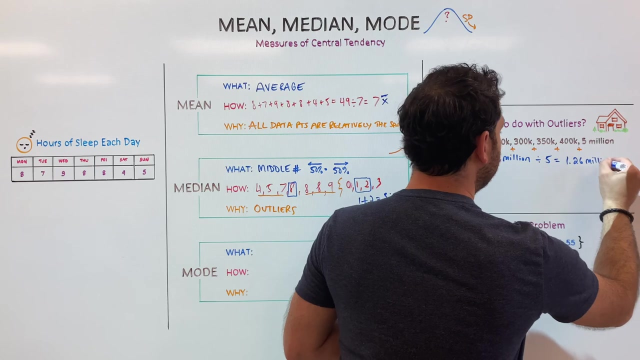 by the number of data points in our data set: 1,, 2,, 3,, 4,, 5 divided by 5.. And what does that equal? $1.26 million becomes our mean, And you remember our symbol right here. 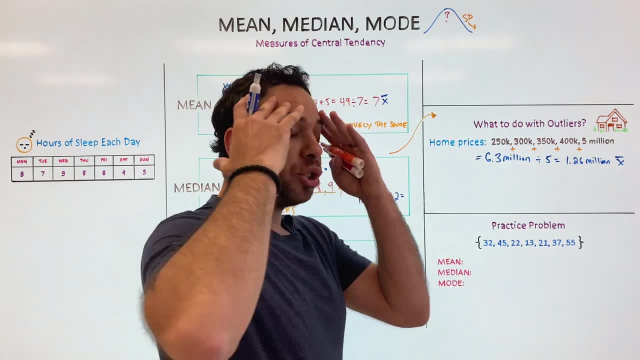 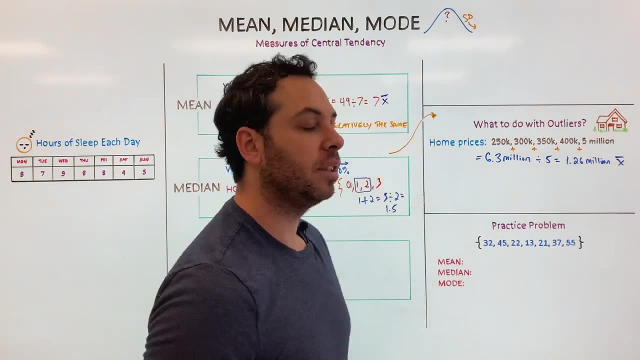 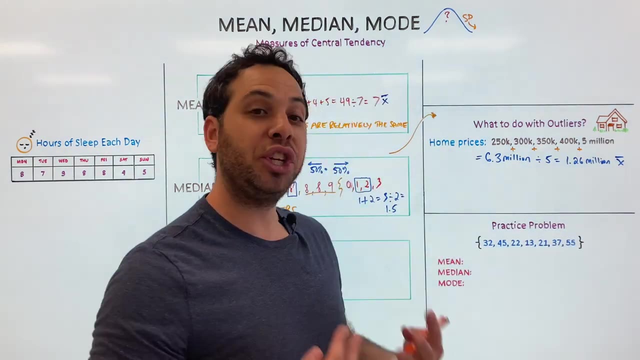 This becomes our mean, And you're thinking: there's no way I can afford a house in this area because the average cost is $1.26 million. What happened? We have one data point that is so far away, that's our outlier that eschews the data, And that's why we don't use the mean. 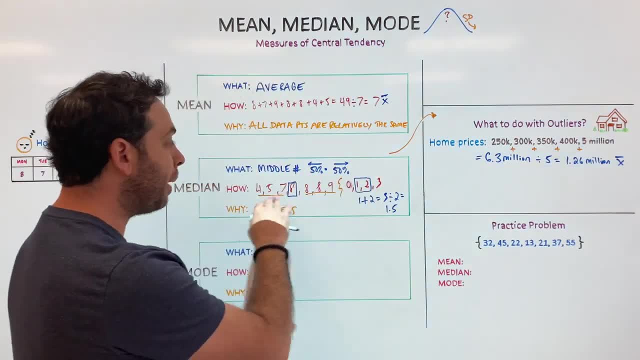 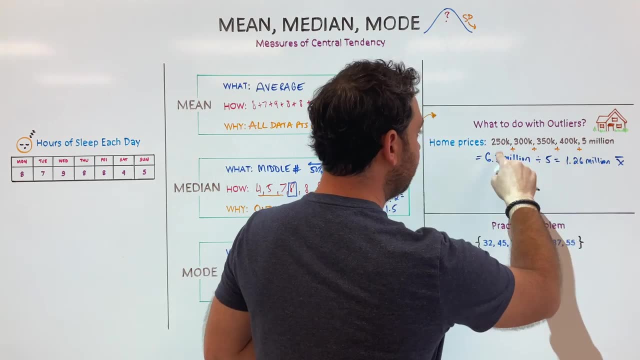 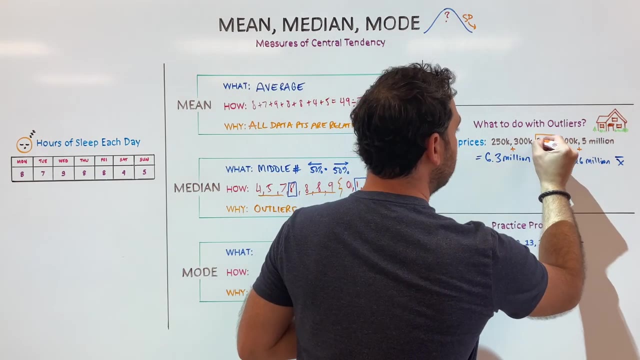 when we have an outlier. Instead, the median is a better representation or a measure of central tenancy in our data. So what would be our median? Well, the numbers already in order: 250, 300, 350, 400, 5 million, What is in the middle, 350,000 is our median. 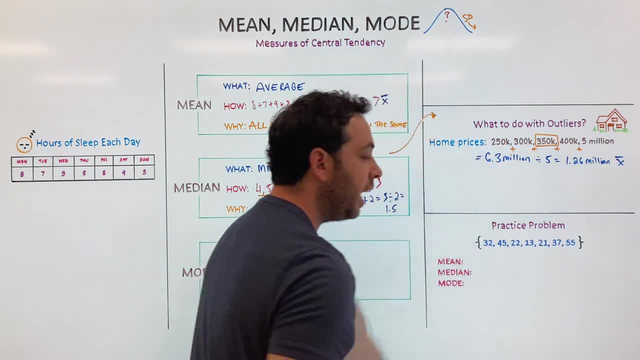 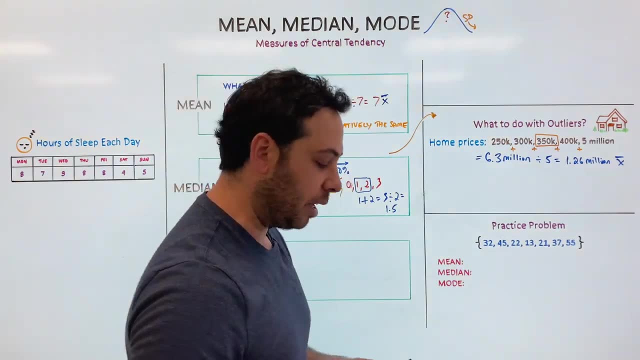 because we have two digits on the right and two digits on the left And because of that it seems like much more attractive. of a neighborhood, 350,000 becomes our median And, by the way, if you look up on Zillow and other websites, home prices. 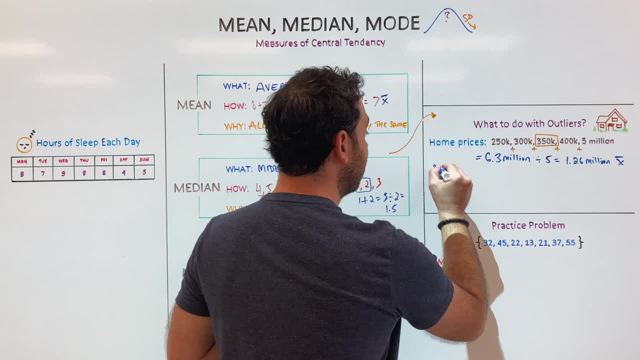 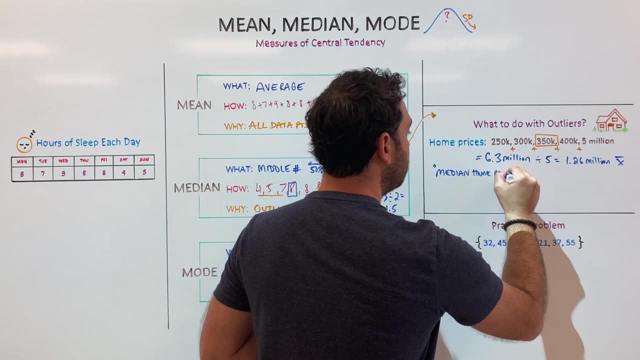 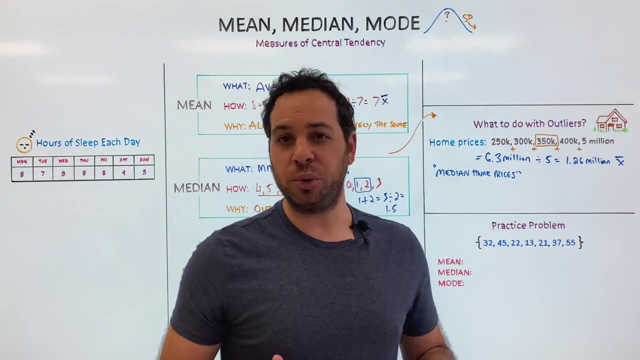 rarely do they say the average or mean. They typically say the median Home prices. They usually talk about the median and not the mean And, by the way, I see this in sports as well. You'll have an average baseball player or basketball player who does something. 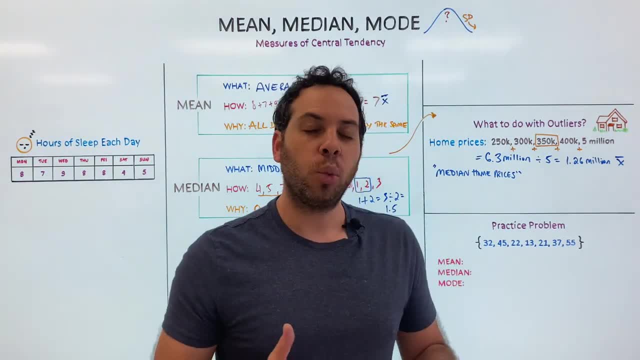 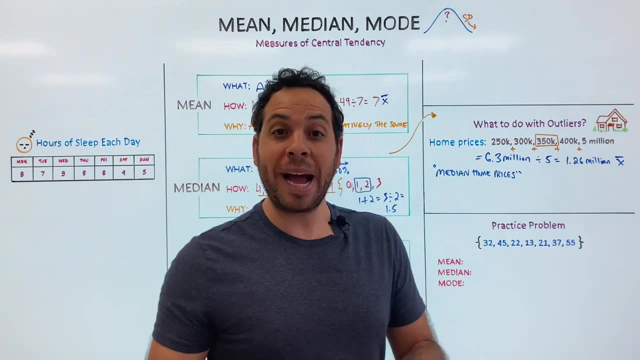 small And then one game. they have a really great game. Well, that skews the data. They're just an average player. So if you have a really good athlete and they have one really good game or one really bad game, I'd recommend to rely on the median, not the mean. All right, So we have. 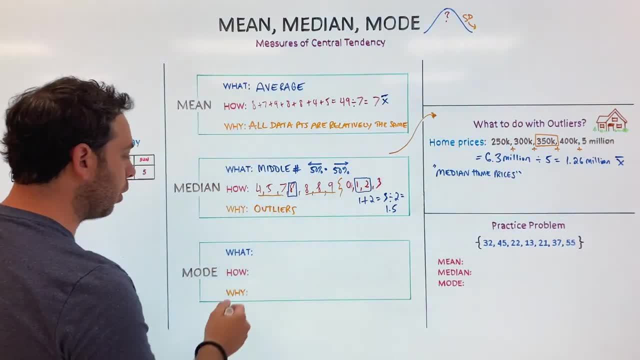 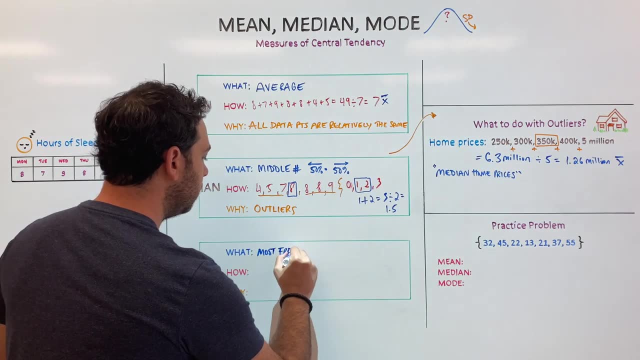 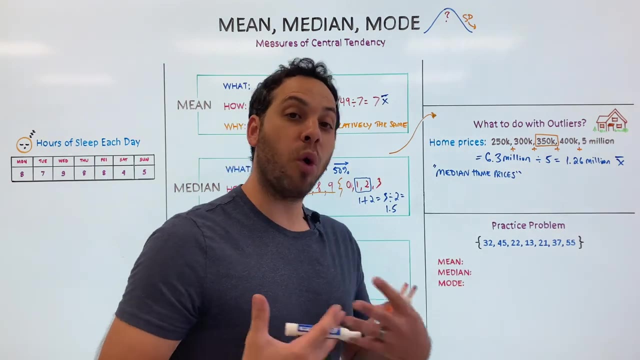 our mean, our median And finally the average, And, by the way, I see this in sports as well. All right, So what is the mode? The mode is the most frequent number, The number, in other words, that repeats over and over again more than the other numbers in our 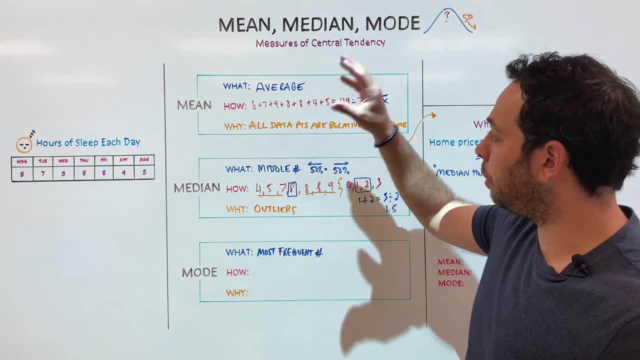 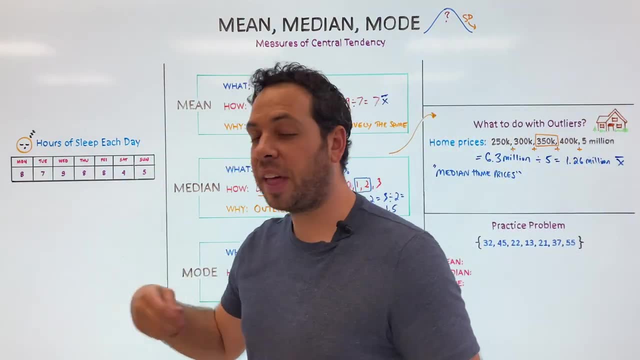 data set. Now there's really no calculation. right In the mean you add up the sum, you divide it by the total data points And then in the median you line them up With the mode. you just look for the data point that occurs the most frequent. 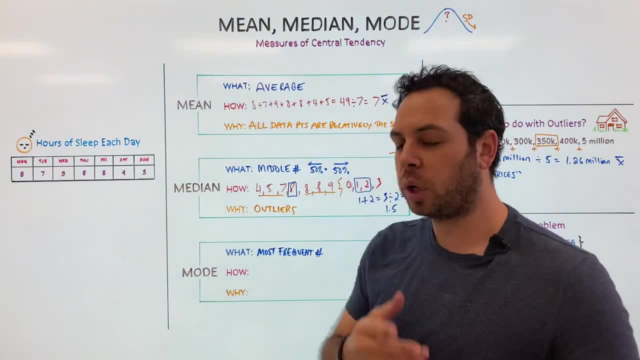 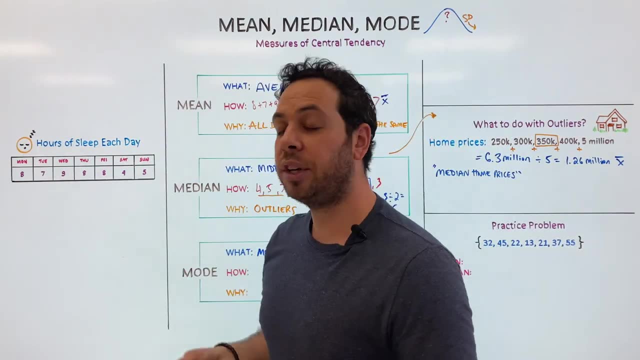 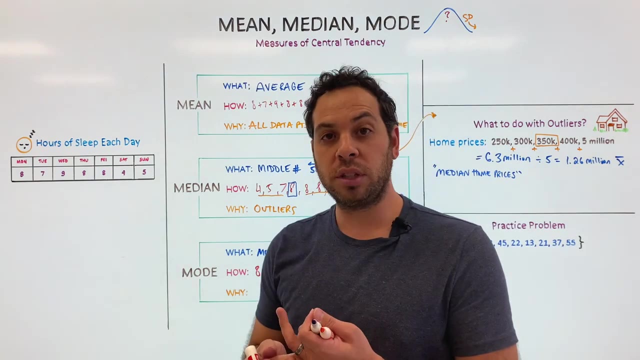 Eight, seven, nine, eight, eight, four, five. So I'll ask you guys, what's our mode? Which number occurs most frequent? The answer: one, two, three. The number eight occurs three times. So eight is our mode, And that's easy. Now can you have no mode? Of course, there could be no mode. 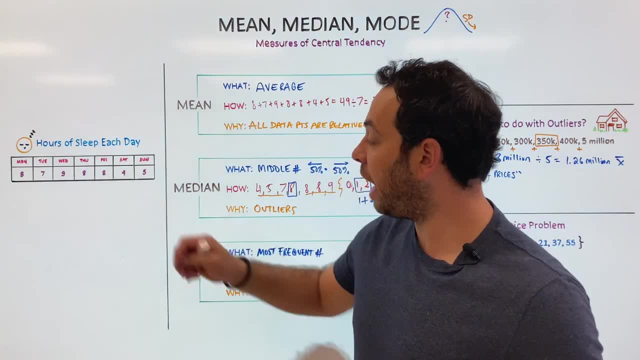 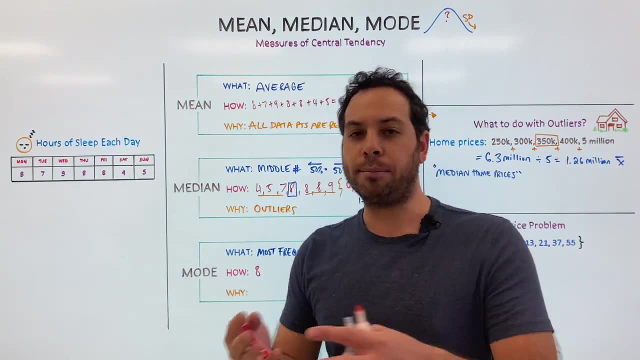 Can you have multiple modes? You can. If the number five repeated twice, then you have, or three times you'd have eight, and five would be our modes as well. So you can have no mode. you have multiple modes and you can have one mode. Now why would we use the mode versus? 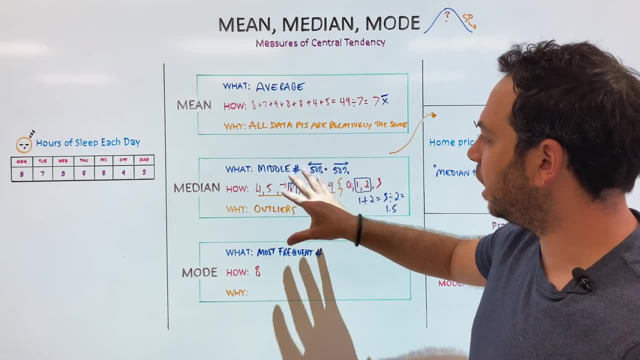 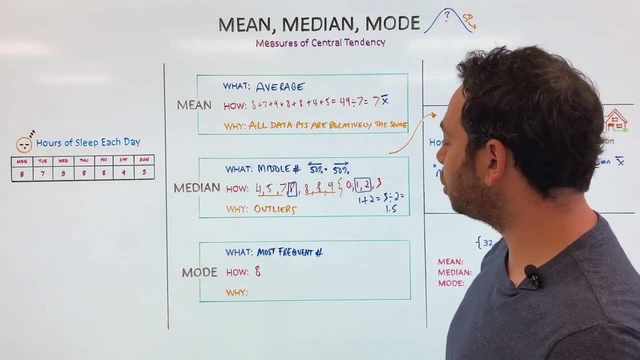 let's say the median and the mean. Well, with the mean and the median you're always getting a number as your answer, But with the mode you don't have to. You see, the mode is the only one of these three measures of central tendency that could give me information about what we call. 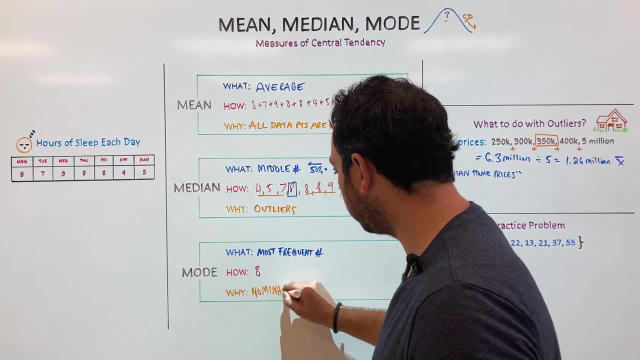 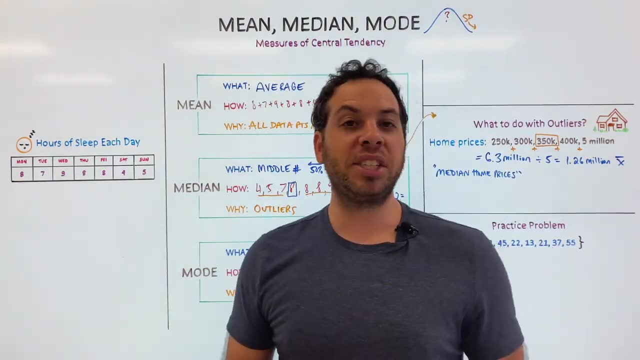 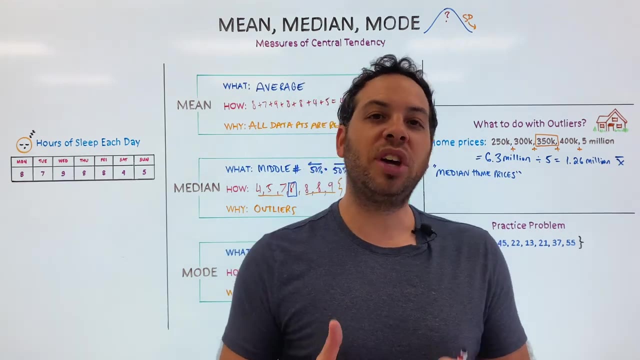 nominal data or categorical data. For example, if I'm doing a study on gender and I'm studying, you know, in my study are more men than women. men is my mode because I have more men than women, So it doesn't have to. 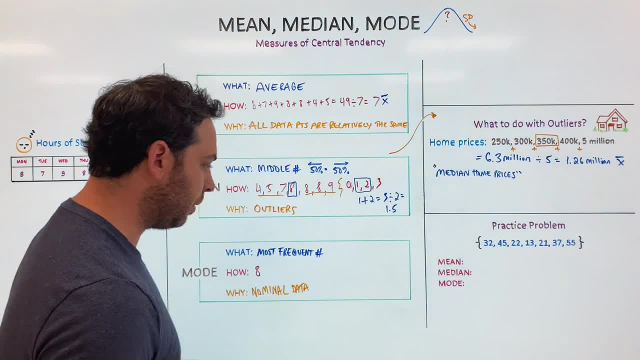 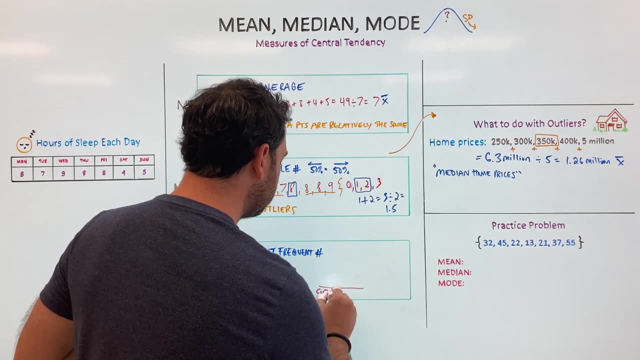 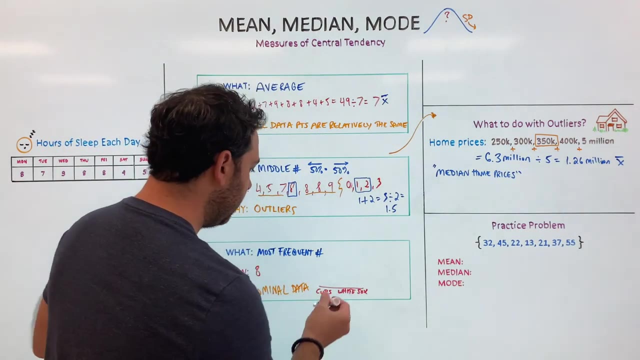 be a number, It could be a category. Here's another example. I'm from Chicago And let's say I'm doing a poll And I want to know: are there more Cubs fans Or are there more White Sox fans in my poll? Okay, And I do my little study And I got, you know, 10 people saying 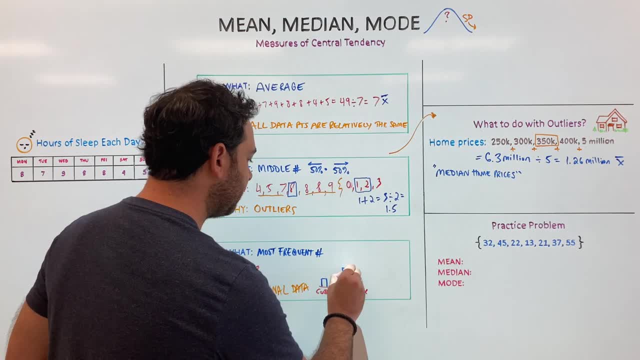 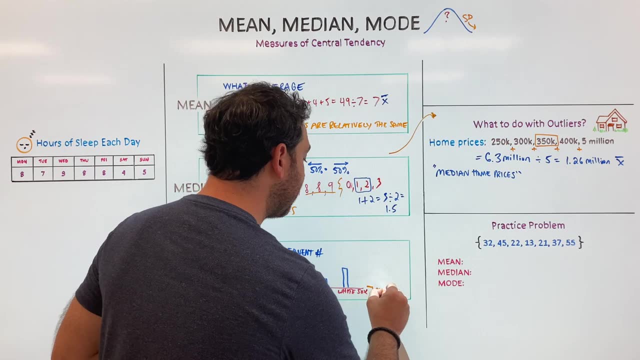 they're Cubs fans And I have 80 people saying they're White Sox And I've got, you know, 20 White Sox fans. What does this tell me? It tells me that my White Sox is my mode. right It's. 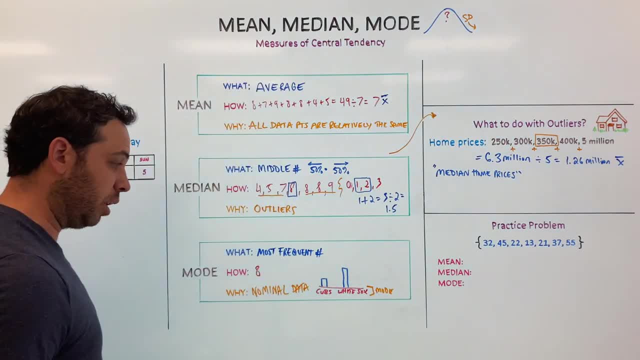 not a number, It's just a category. Okay, So White Sox is my mode And if you can't tell, yes, I'm a White Sox fan. That's why we have more fans than the Cubs. All right, So we have our, mean, our. 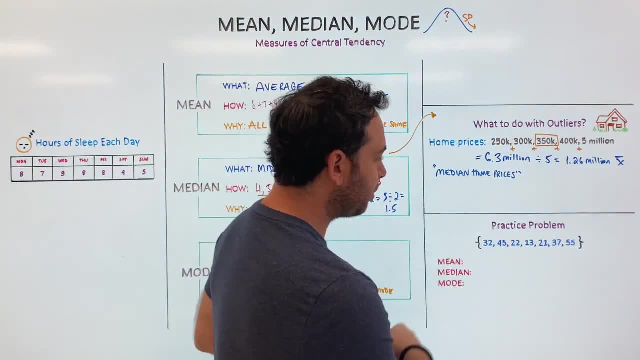 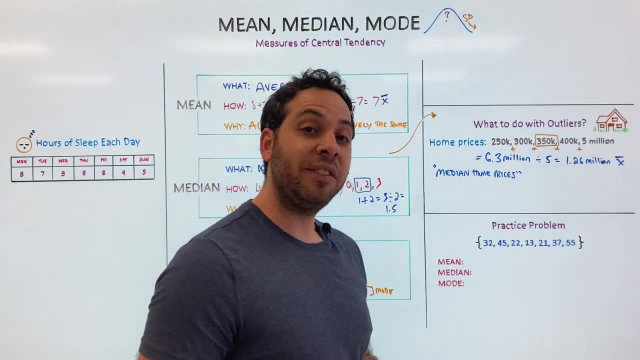 median and our mode. All right, guys, before you leave, I do have a practice problem for you, And here is our data set. Your responsibility is to try to find the mean, the median and the mode. Now, I'm not going to give you the answer here, But if you scroll,